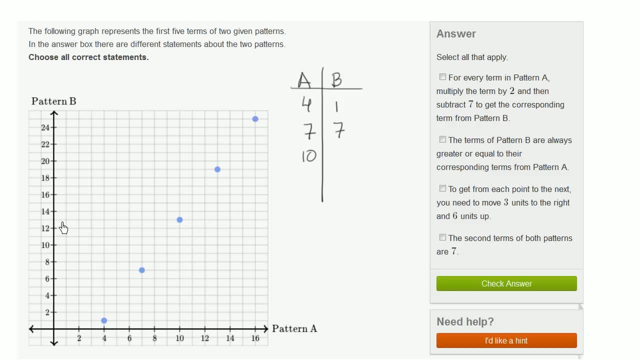 Third term: pattern A is 10, and pattern B is 13. And then fourth term: pattern A is 13. And pattern B is 19.. And then, finally, fifth term: pattern A is 16. And pattern B is 25.. 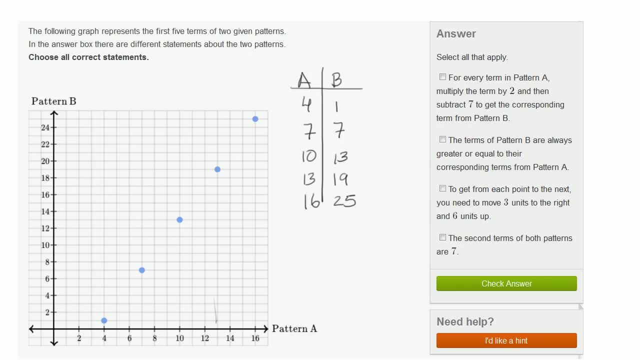 Now, before even looking at these, let's see what we can think about these patterns here. So it looks like pattern A starts at 4, and it increases by 3 every time. To go from one term to the next, you just have to add 3.. 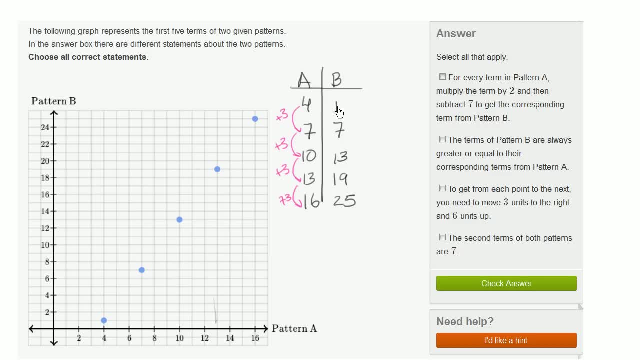 Now, what about for pattern B? Well, pattern B starts at 1, and every term here it looks like you're adding 6.. When pattern A increases by 3, and we're moving in the horizontal direction, based on the fact that pattern A is represented on the horizontal axis. 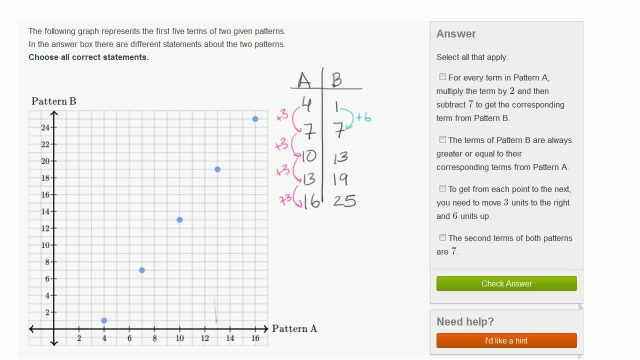 we're gonna move up 6 in the vertical axis and we see that here. Pattern A increases by 3 from one term to the next, and when that increased by 3, pattern B increased by 6 from one term to the next. 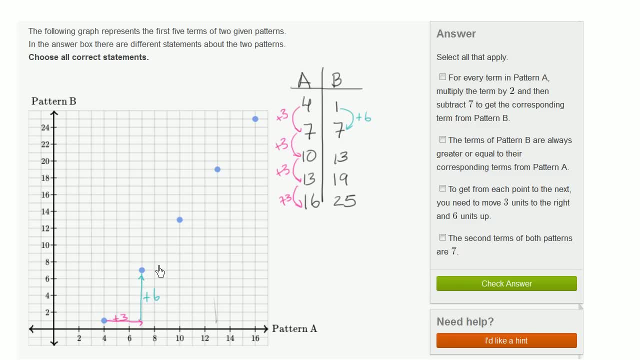 to the next. Pattern B, increased by 6 from one term to the next, And we see that it keeps doing that. Now let's think about what we have over here to see which of these statements actually apply to this. For every term in pattern A, multiply the term by 2. 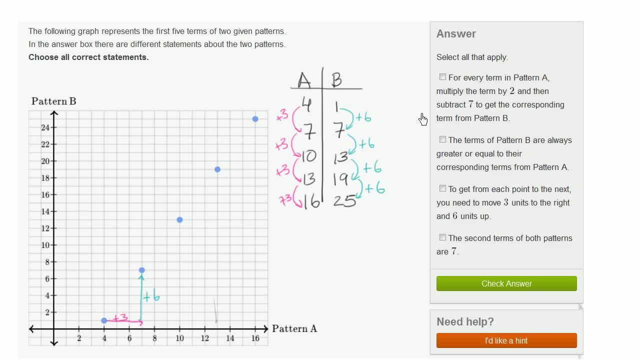 and then subtract 7 to get the corresponding term from pattern B. So let's see if that holds up. So according to this, if this was true, I should be able to take this, multiply by 2, and subtract 7 and get that. 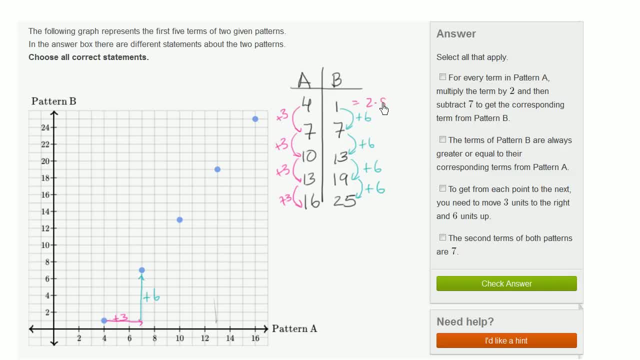 So let's see: is 1 equal to 2 times 4 minus 7?? So 2 times this number, 2 times 4 minus 7.. Well, 8 minus 7 is equal to 1.. Is this, right over here, equal to 2 times this 7 minus 7?? 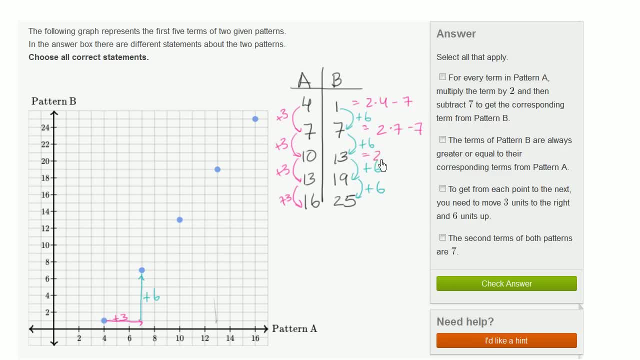 Well, yeah, it's equal to 7.. Is 13 equal to 2 times 10?? 2 times 10 minus 7.. Yeah, 20 minus 7 is 13.. Is 19 equal to 2 times 13 minus 7?? 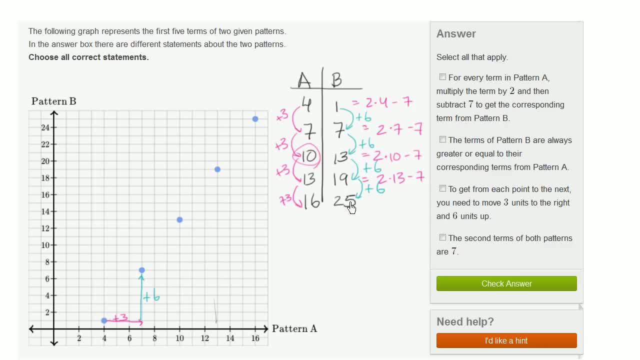 26 minus 7 is 19.. Is 25 equal to 2 times 16 minus 7?? Well, 32 minus 7 is 25.. So this first statement checks out, For the corresponding term, the value of pattern B. 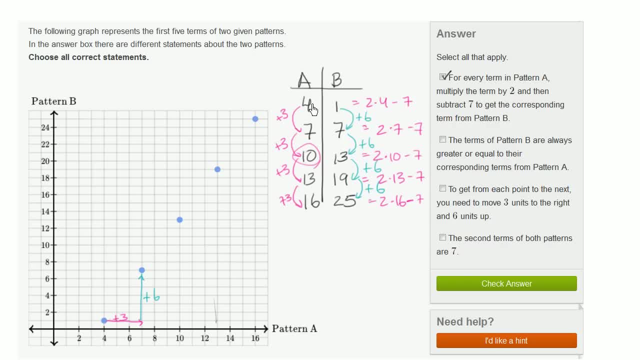 is 2 times the value of pattern A minus 7.. Now let's look at the second one. The terms of pattern B are always greater than or equal to their corresponding terms from pattern A. Well, no, that's not right. It's true for a couple of scenarios. 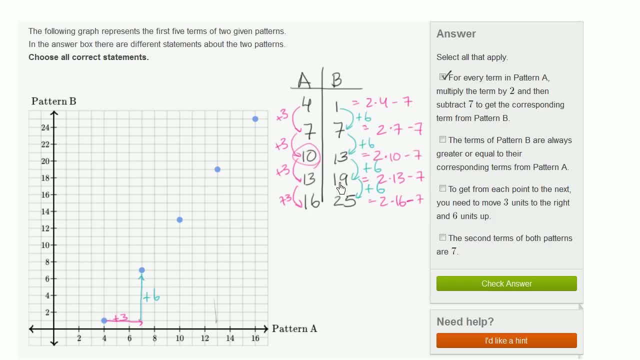 Here for the second, third, fourth and fifth terms. pattern B is equal to or greater than pattern A, But for the first term it's not true. Pattern A is greater. So this is not right To get from each point to the next. 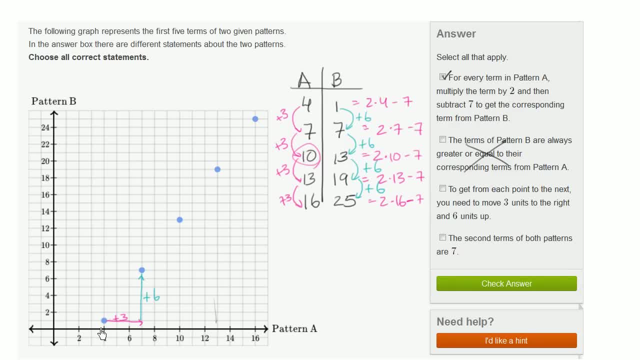 you need to move 3 units to the right and 6 units up. Well, that's exactly what we talked about. From one term to the next, pattern A, along our horizontal axis, we increase by 3, while pattern B, which is plotted, 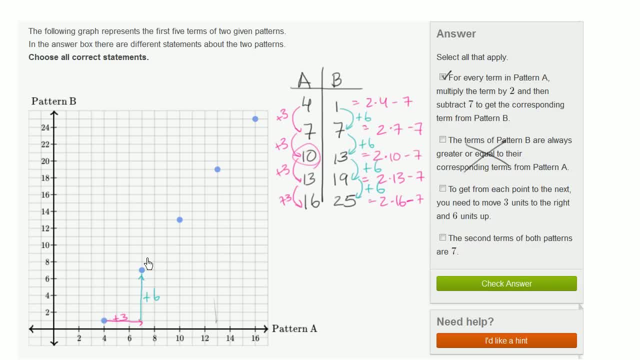 on our vertical axis by 6.. So you move 3 to the right and 6 up. So that is right. The second terms of both patterns are 7.. Well, yeah, we see that right over here. The second terms are 7.. 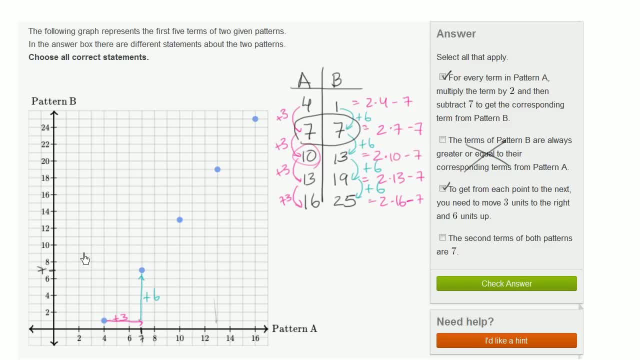 We have 7 here and we have 7 there, And so that is right as well. So the only one that doesn't apply is this second one. This is not right. 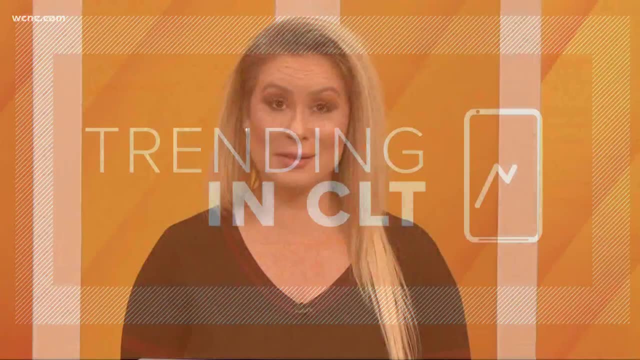 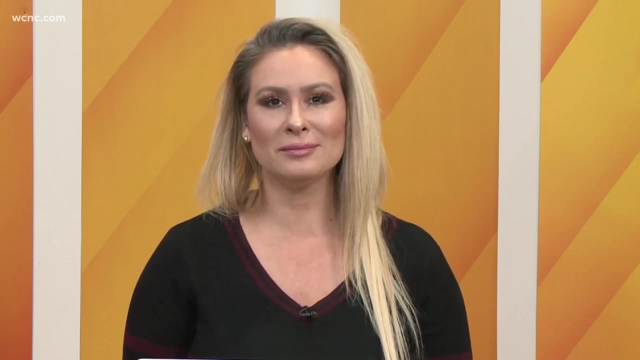 All right, let's talk what's trending. There's a lot of buzz about ticket prices for the Charlotte Football Club, so everyone was excited. Soccer is coming to Charlotte. well, It is the first team in the league that's requiring you buy personal. 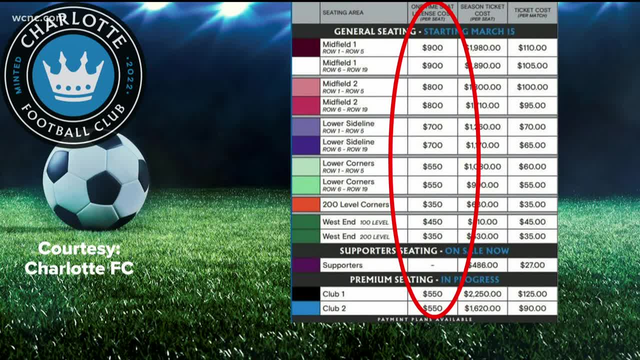 seat licenses- so PSL's- in order to then buy season tickets. It's a one time fee, It's anywhere, though, from $350 to 900 bucks, And then, on top of that, you have to pay for the season tickets- which, by the way,